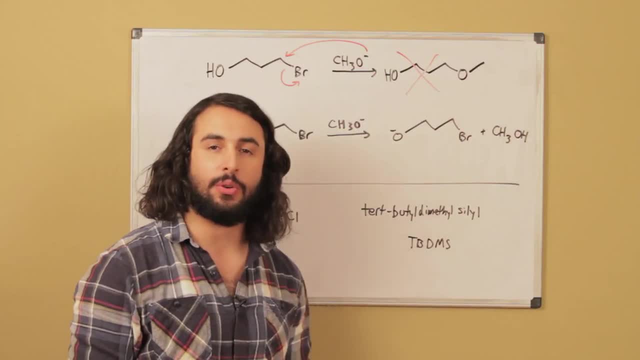 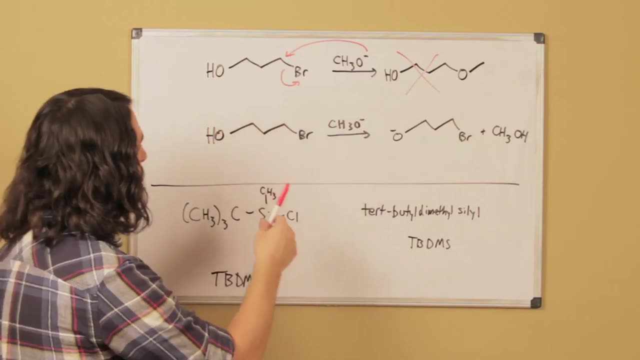 but actually this is no good. it's not going to go SN2, and let's talk about why. because not only is this a good nucleophile, it's also a very strong base, and so the thing is because we have a hydroxyl group right here. 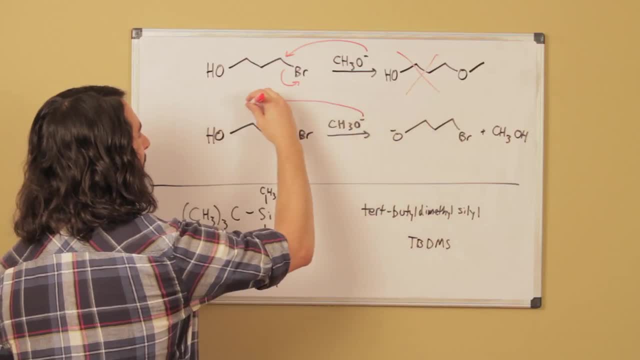 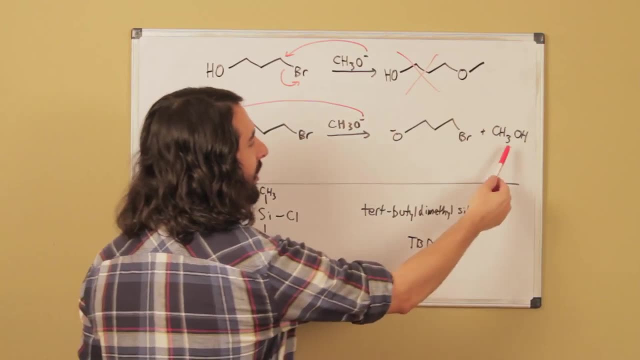 this is just acidic enough that a strong base is. actually it's just going to do an acid-base reaction. so this alkoxide, this methoxide, is going to pick up that proton to form methanol and then we're going to have the alkoxy group right there. 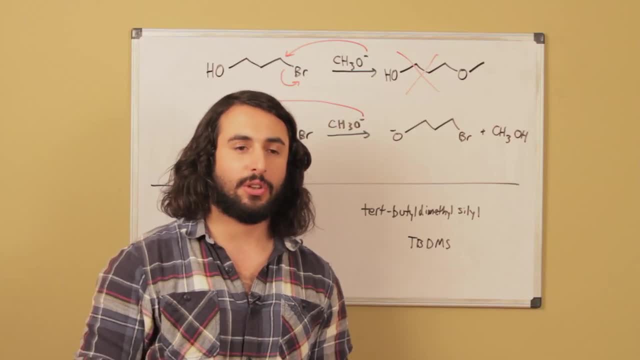 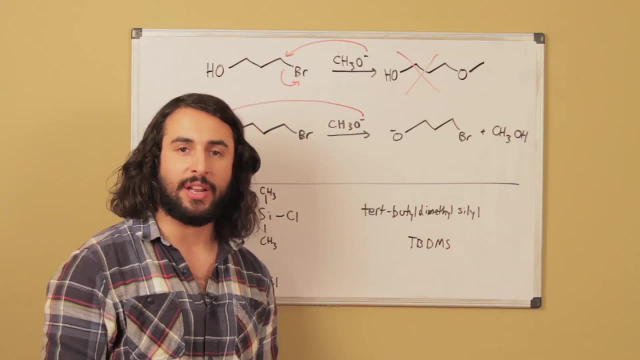 we've ruined our nucleophile, we're not going to get any SN2, and so everything is terrible. but what we come to understand is there's ways to manipulate our substrate so that we can do the SN2 that we planned, and the way that we can do that is by protecting the hydroxyl group. so if we protect that, 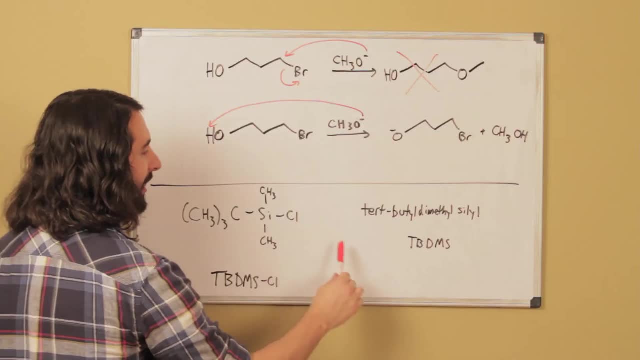 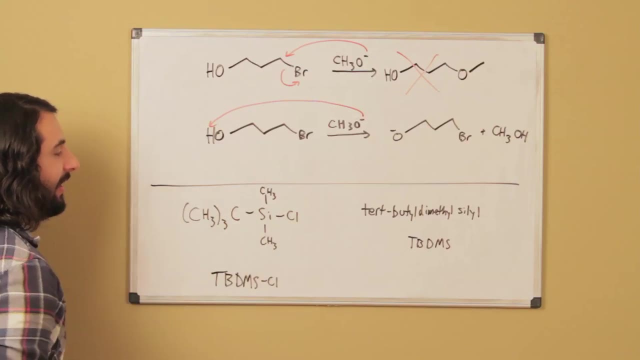 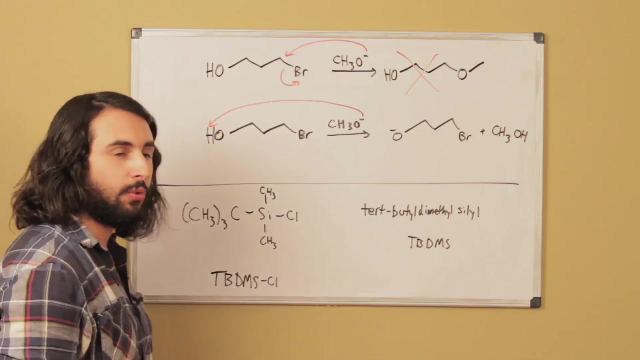 alcohol using TBDMS group. this is a tert-butyl-dimethyl-silyl, because this is a tert-butyl, right here a dimethyl, and then silyl refers to a silicon atom. this is actually going to work as a protecting group for that hydroxyl group. 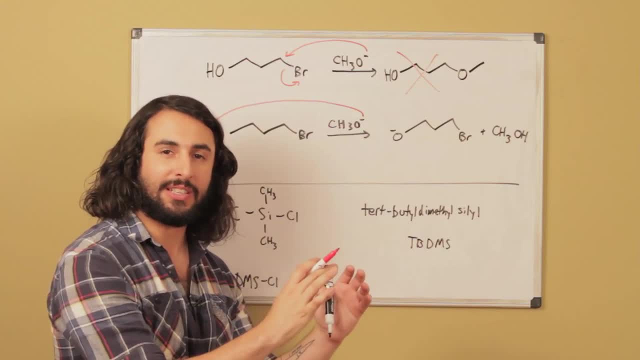 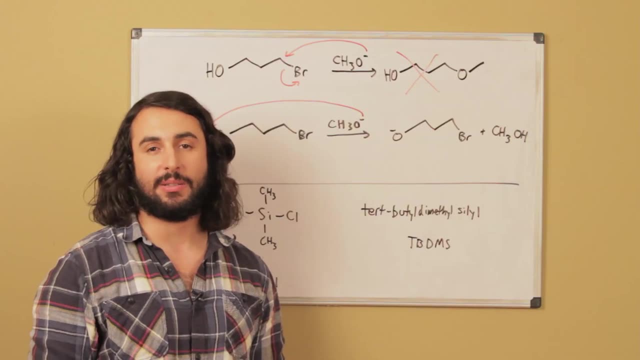 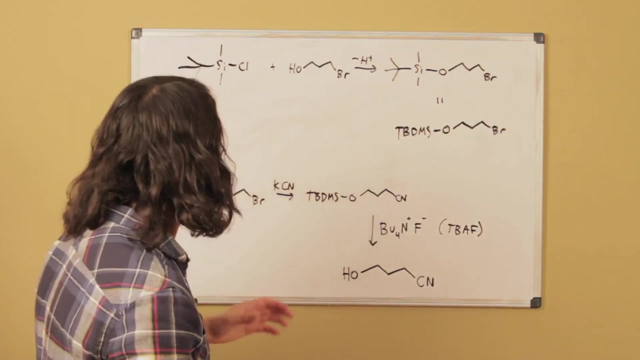 so it will temporarily shield it from any unwanted acid-base chemistry. we can do the SN2 we wanted and then deprotect it and get it back to normal. let's take a look at how this mechanism works. so let's take a look at how this mechanism works. so let's say we have our substrate that we were. 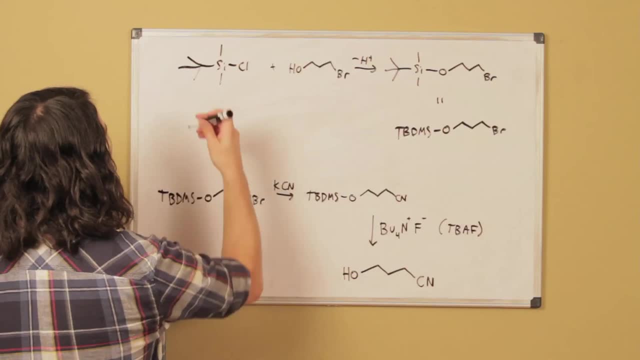 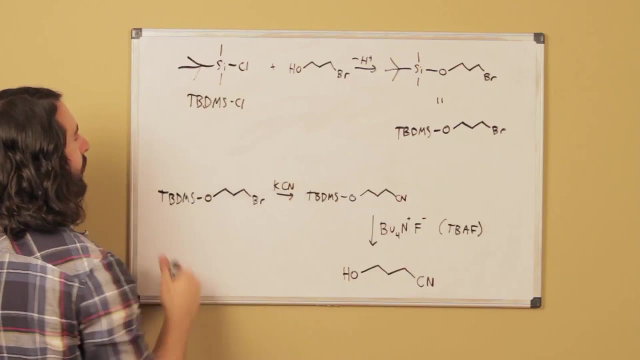 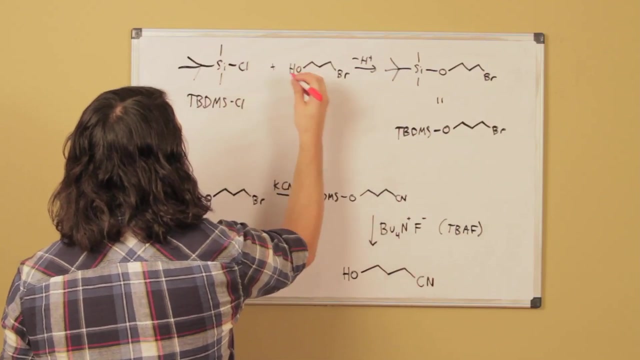 looking at before. and then here is our. this is called TBDMS-Cl. we've got our tert-butyl-dimethyl-silyl group there and then the chloro group there. ok, so what's going to happen is the. the oxygen atom is more labile than the. 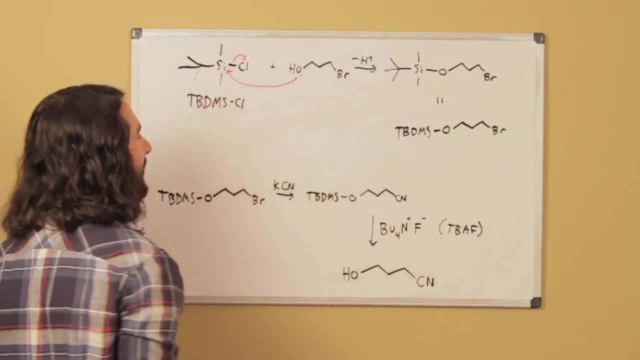 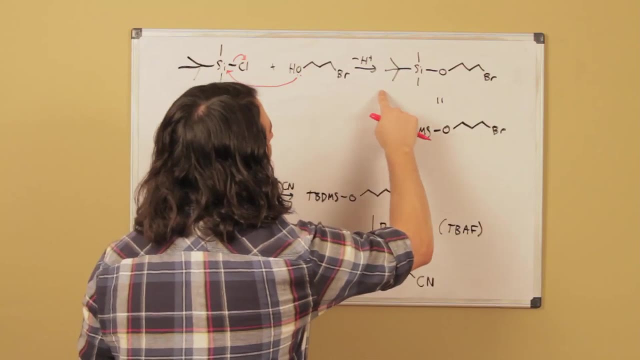 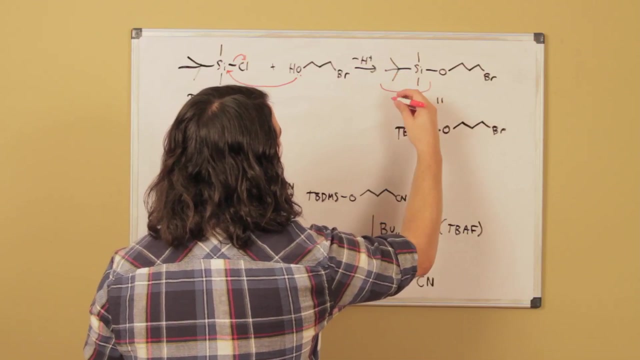 chlorine atom, so this is actually going to be able to displace the chlorine. the oxygen is more electronegative, so it is actually going to be able to attack the silicon atom and displace the chlorine. so now we have this whole TBDMS group on that substrate. so remember this is TBDMS, so we can. 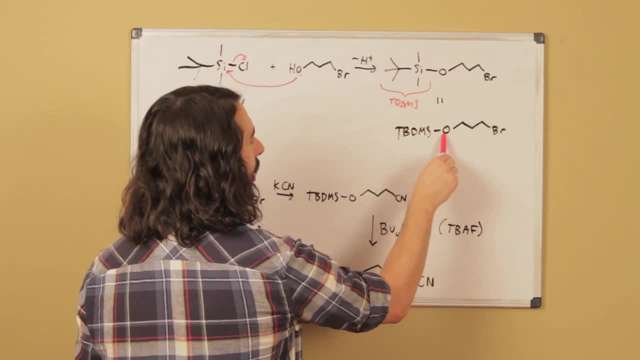 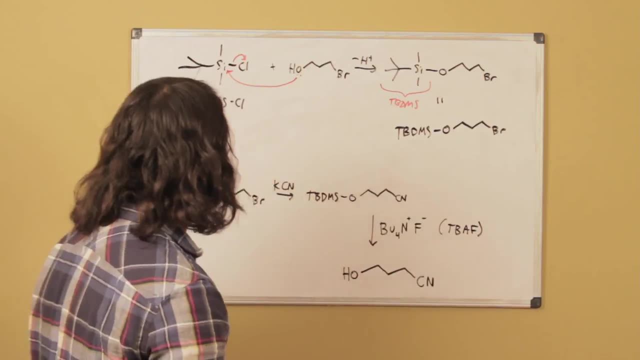 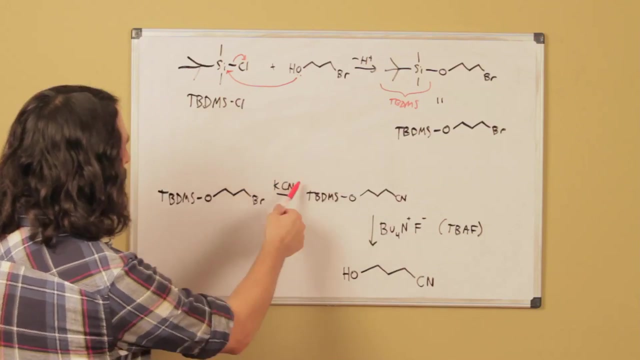 actually abbreviate that as TBDMS bound to the oxygen atom and then the rest of the substrate. now here's what's very interesting about: about putting this protecting group on the hydroxyl. remember how before, whether it was some base or whatever it was- we were worried about an acid-base reaction with the 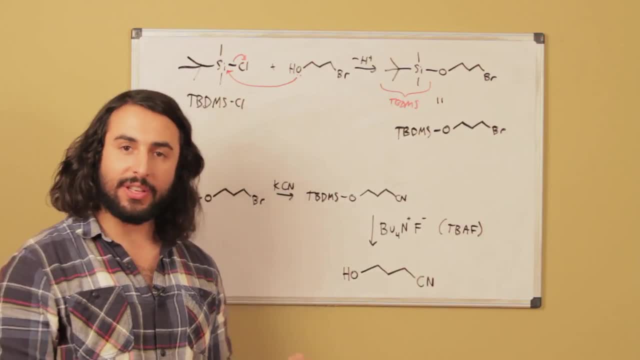 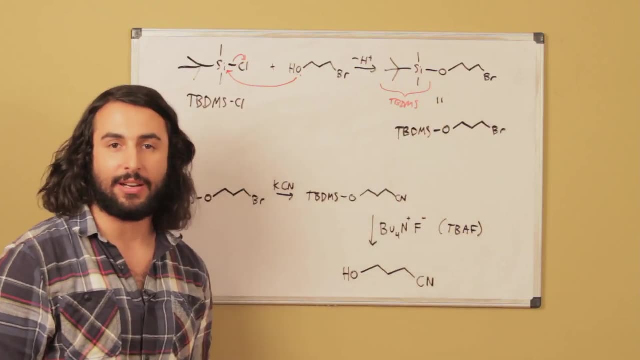 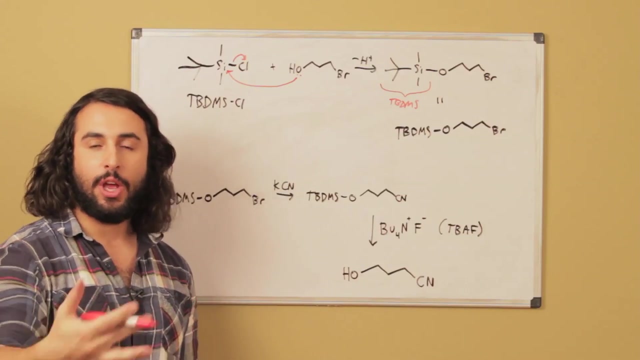 nucleophile and that hydroxyl proton. well, guess what? there is no longer a hydroxyl proton. this oxygen is not bound to hydrogen anymore, it's bound to a silicon atom. so there is no longer a proton that is acidic enough to react with whatever base or nucleophile we might be trying to use to do an SN2 reaction. so now, 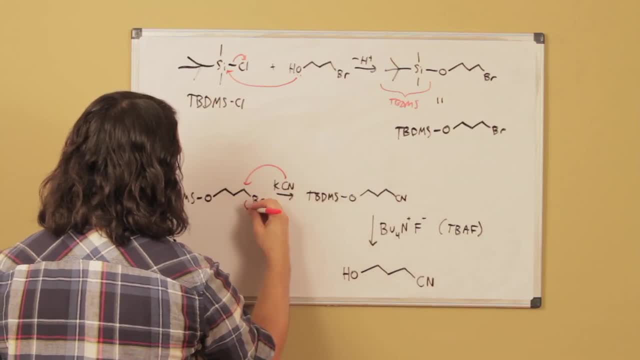 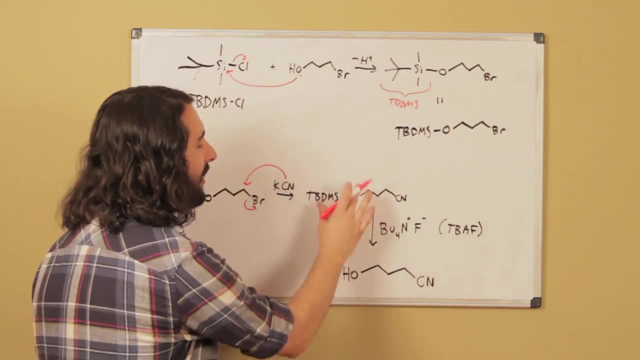 there's no worries, let's do an SN2 reaction. let's say KCN, whatever it is doesn't matter. so here we go, we did our SN2 reaction. so the SN2 reaction is now complete without any interference from the hydroxyl group. now that we've 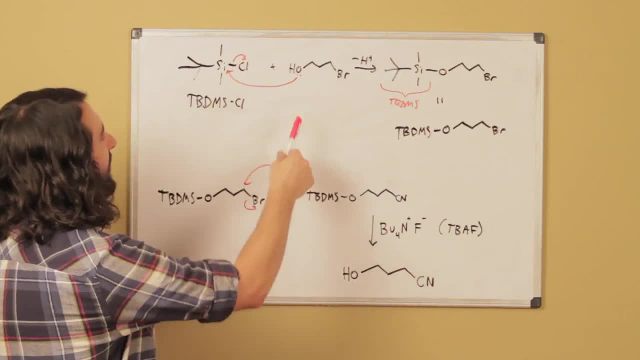 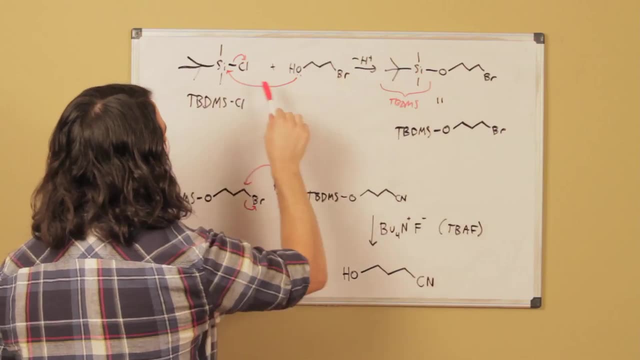 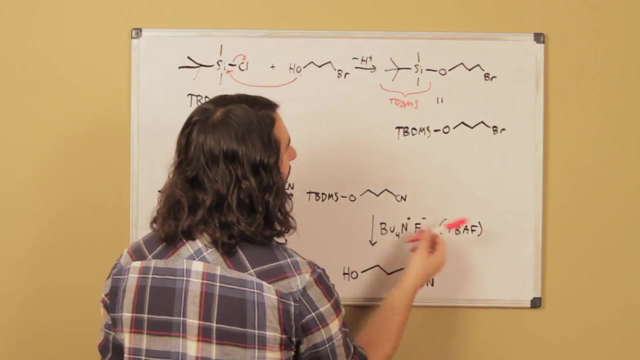 achieved that. we do want to get our hydroxyl group back. so remember how we said that oxygen was more labile than silicon, so the oxygen silicon bond was able to replace the silicon-chlorine bond. well, now this fluoride is more labile than even the oxygen. so a fluoride can come in here, boom, attack the. 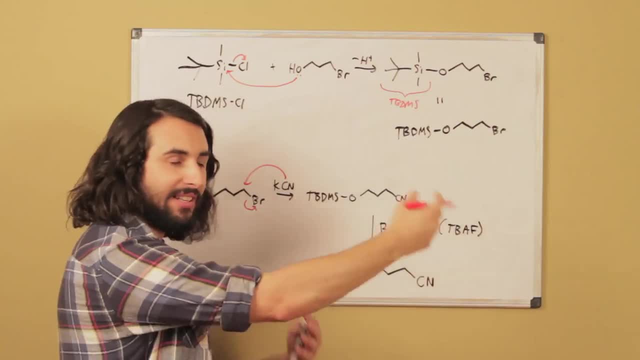 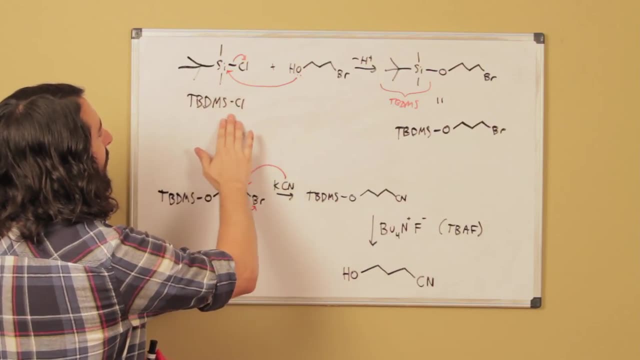 silicon. kick that off, then that's going to protonate. let's say it gets a proton from solvent somewhere and then we're going to get our hydroxyl back. so all we did was we used TBDMS-Cl to protect the hydroxyl group. this is now protected. 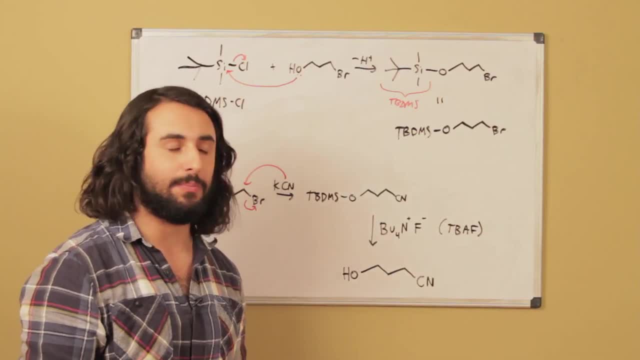 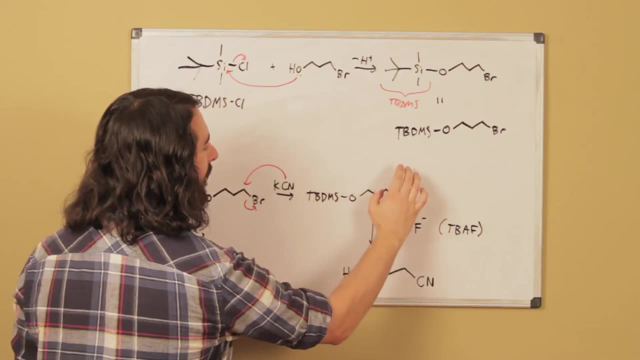 there is no hydroxyl proton there to participate in any acid-base reaction. we use that protected version of the substrate to do whatever SN2 we wanted. doesn't matter what it was, we achieved the SN2, once we did that, we deprotect. 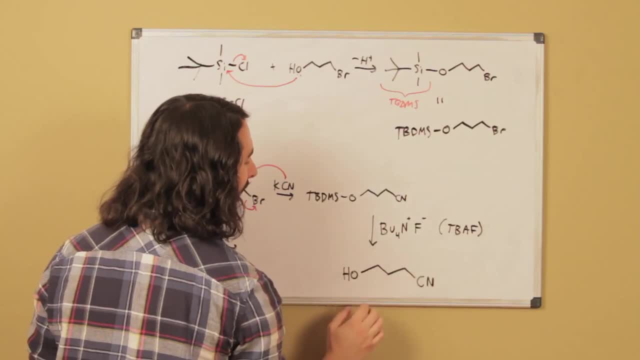 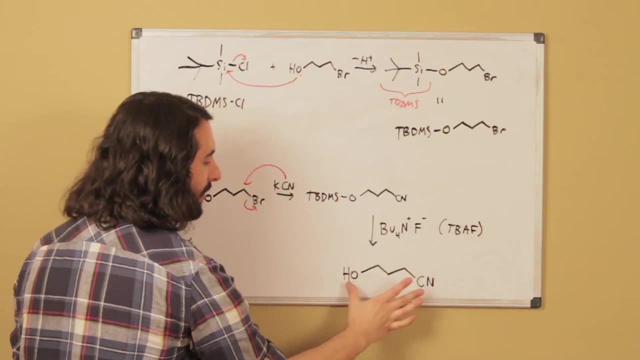 with TBAF. this is tetra butyl ammonium fluoride, and that's because the fluoride can then displace the silicon-oxygen bond. oxyanion gets protonated from solvent and there we go. we have our deprotected alcohol back to normal, and 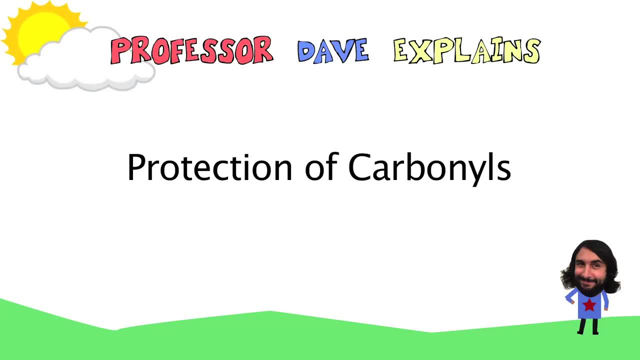 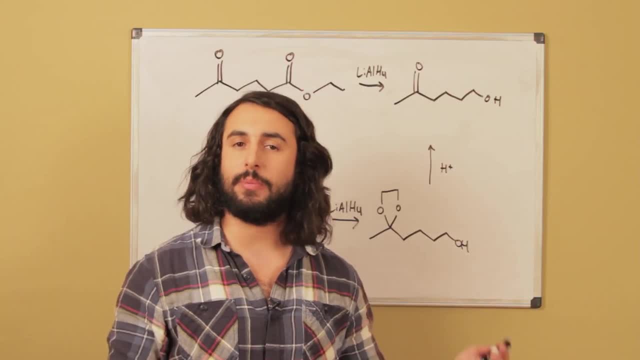 with the SN2. that we wanted to do achieved. now we looked at protecting groups for hydroxyl groups, but there's protecting groups for pretty much any functional group you can think of. so let's look at one more. let's look at a protecting group for an aldehyde, or 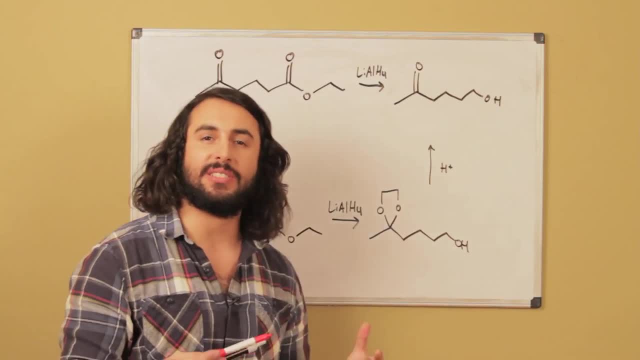 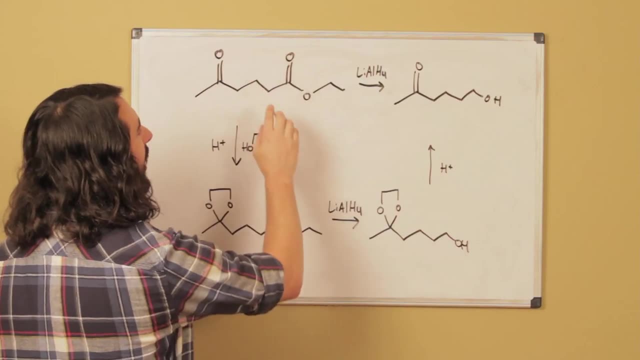 ketone. so let's say we want to achieve- once again, this is always about some kind of transformation we want to achieve- but there's a different functional group that's going to mess it up. so let's say we have this substrate here and we 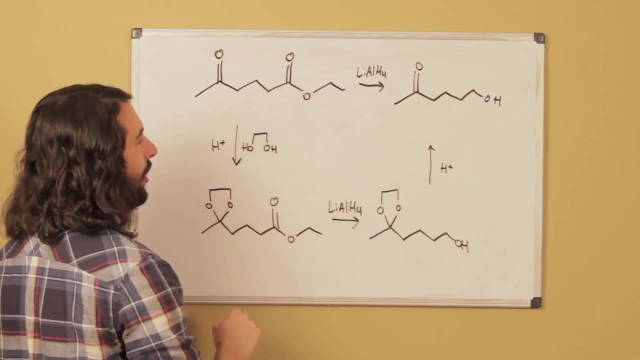 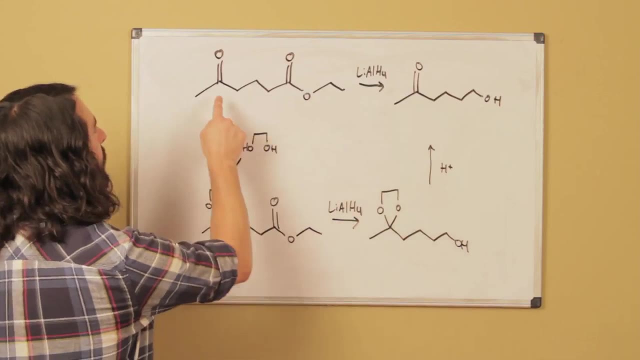 want to specifically reduce this ester. we want to reduce this ester to the primary alcohol. we really want to do that. for whatever synthetic pathway we're doing, who cares why? but here's the problem. we've got a ketone right there. there's no way we're gonna get lithium aluminum hydride to selectively reduce. 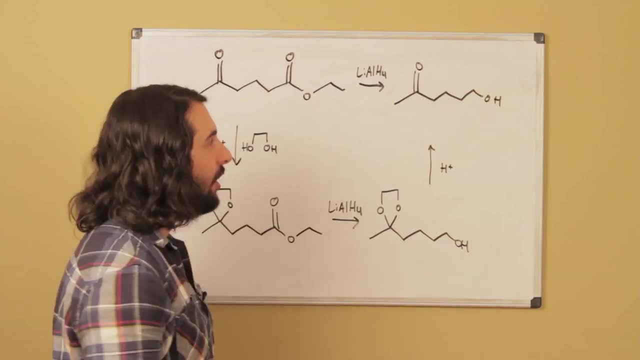 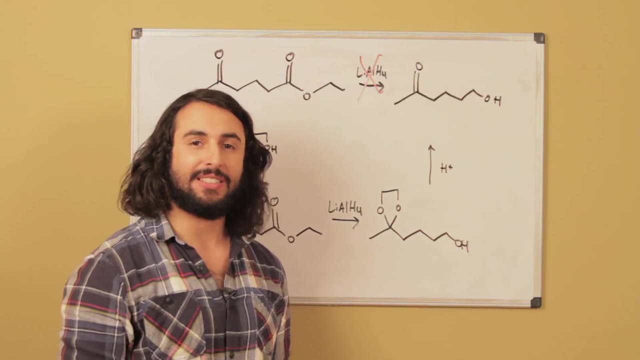 the ester and not the ketone. it's going to reduce whatever it sees first. so we wouldn't get this product and this reaction is not going to work. but here's the thing: what if we protect that carbonyl, specifically the ketone? so what we're going to do is we can react in acidic conditions with 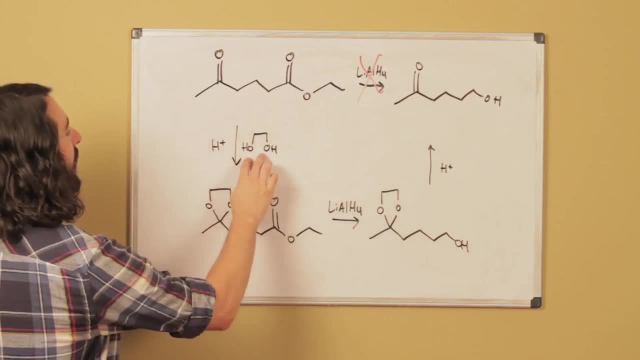 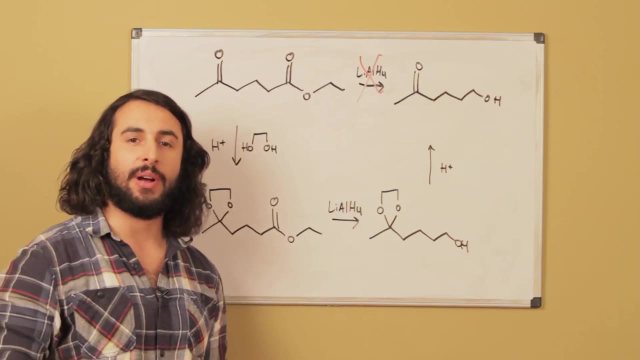 this 1,2-ethanediol. we have this vicinal diol here now. I'm not going to write out the whole mechanism explicitly because this has to do with acetal formation and you can check out my acetal tutorial to see this very. 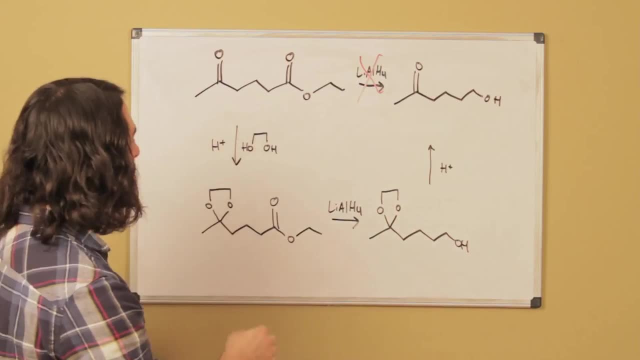 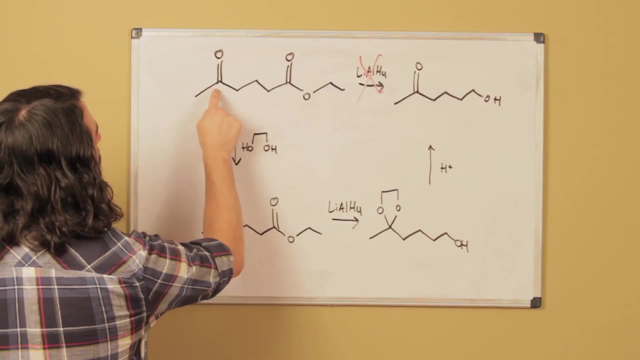 explicit mechanism, but let's just say that that mechanism occurs and what ends up happening is we get this acetal here, okay, and so the reason that this attacks over here, not over there, is because this is a little bit more electrophilic at the time. 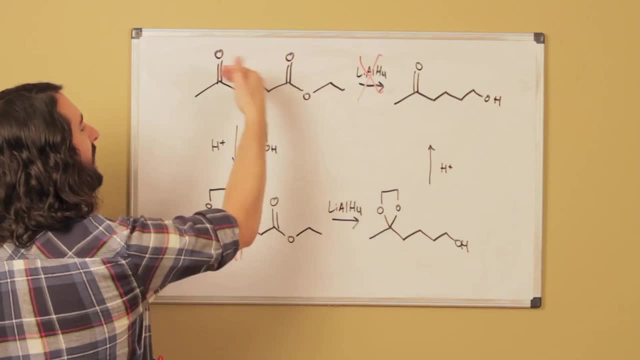 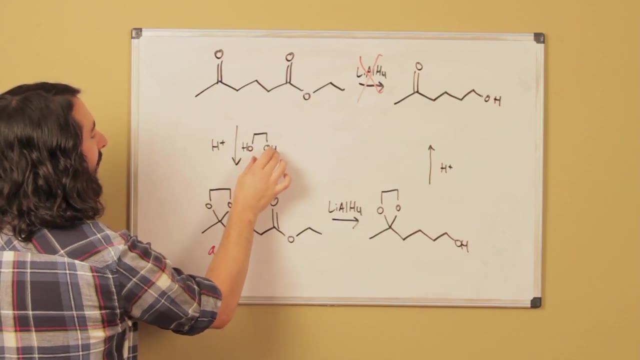 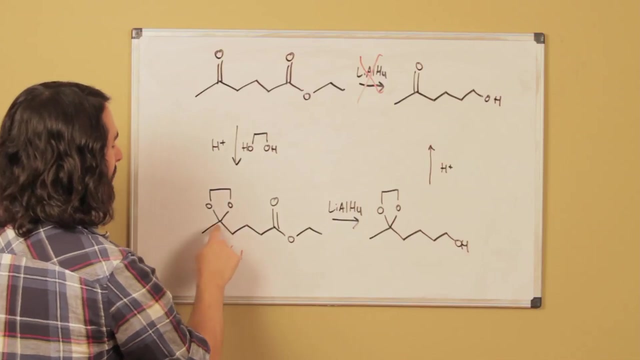 because this carbonyl carbon is receiving extra electron density from the lone pairs on that oxygen, so this is less electrophilic than here. so this ethanediol will explicitly undergo acetal formation at this site. now the reason that this is useful is because this carbon still has two 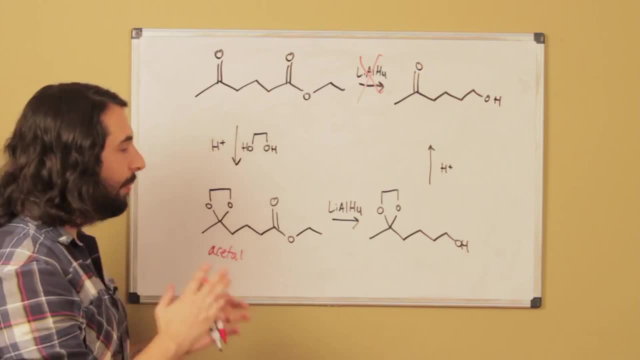 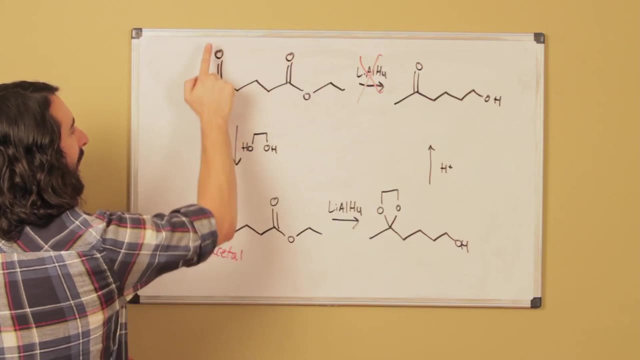 carbon-oxygen bonds, so we would still consider it electrophilic. but if you look at the vectors, the dipole on this bond, it has two carbon-oxygen bonds in the same direction. so that is why a carbonyl carbon is very electrophilic, because it 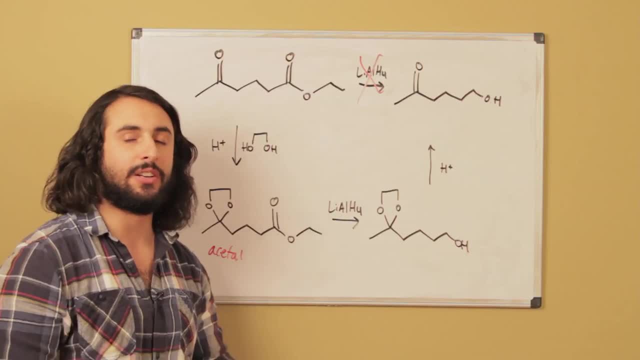 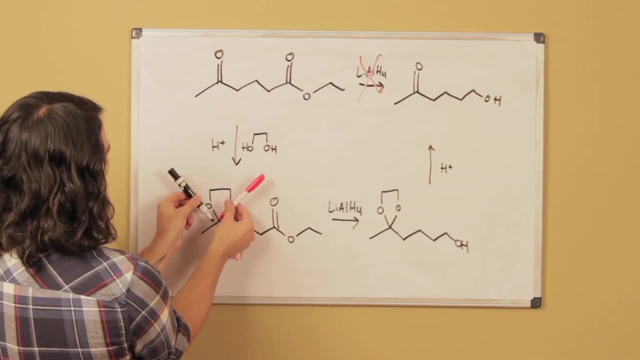 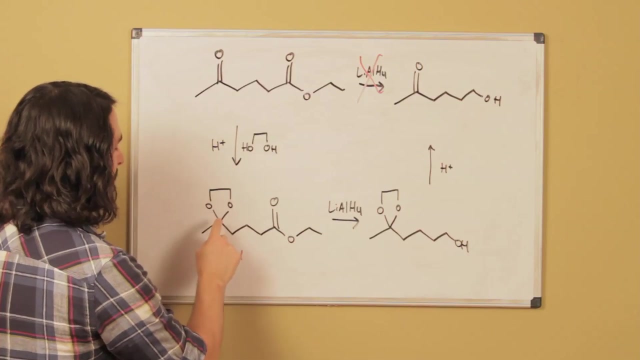 has two carbon-oxygen bonds. it has its electrons being withdrawn away from it by two bonds and in the same direction. but if we do this, then it becomes two vectors that are like this, and so they're not any longer unidirectional. this greatly reduces the electrophilicity of that carbon.